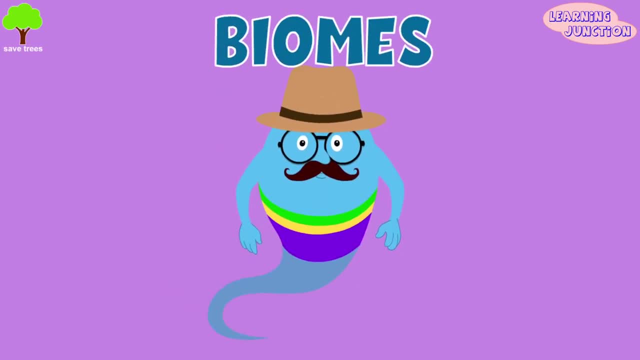 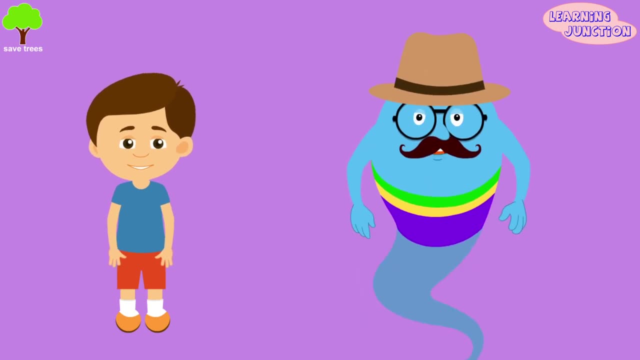 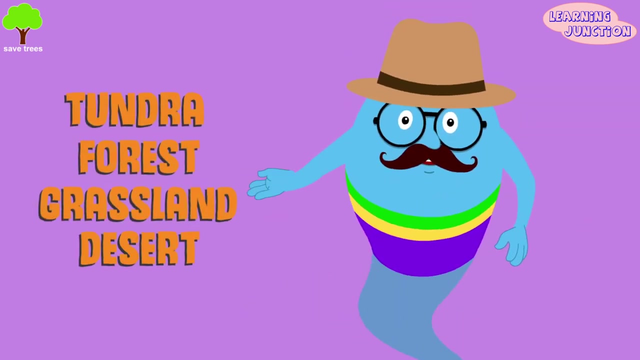 Hello friends, Today we'll learn about the biomes. A biome is a huge region of Earth that has a certain climate and certain types of organisms. Four major biomes are tundra, forest, grassland and desert. Let's learn about each one by one. 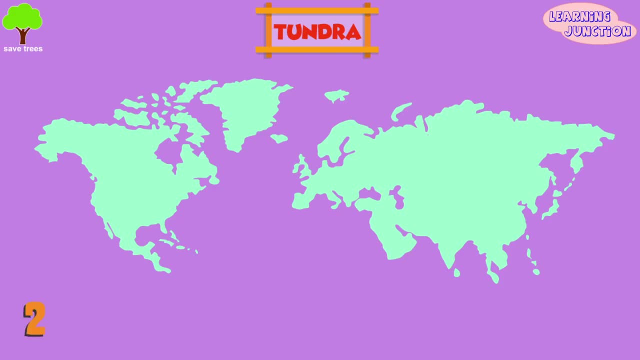 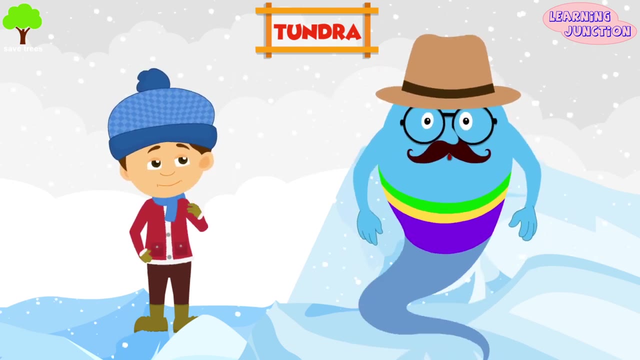 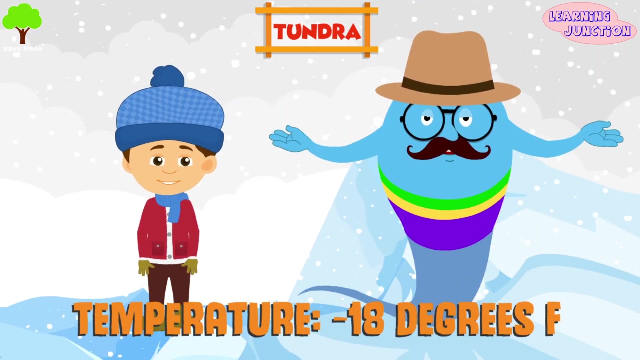 At first, the tundra biome. Around 20% of the Earth's land surface is covered with this biome. The tundra biome is the coldest among all the biomes. The average temperature in the tundra is approximately minus 18 degrees Fahrenheit. Some lichens and small shrubs flourish in the 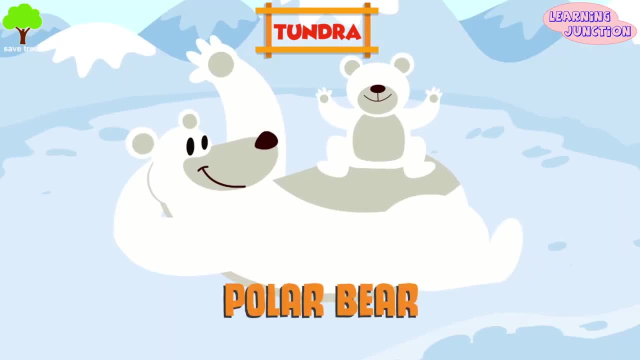 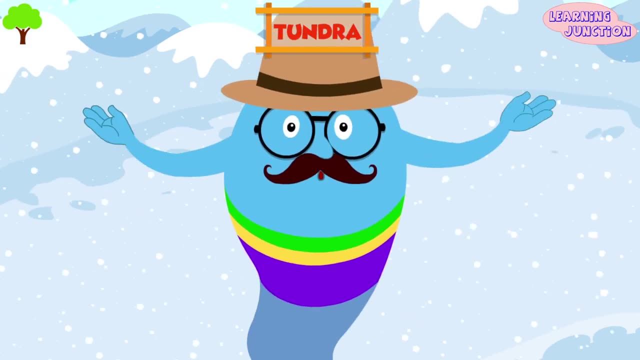 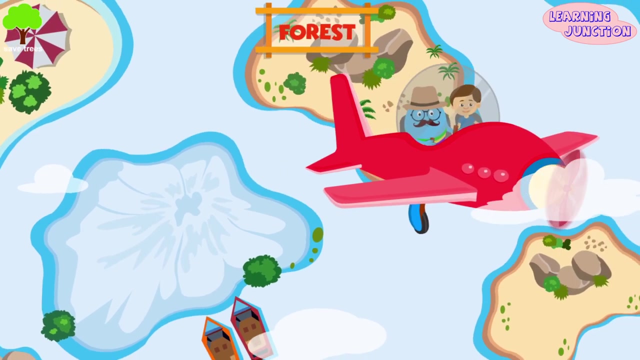 Arctic tundra. Careful polar bears live in the tundra. They are the largest carnivorous land mammals on Earth. Hmm, due to harsh climate, people do not prefer to live here. Now we're going towards the forests. There are three types of forest biomes: the rainforest, 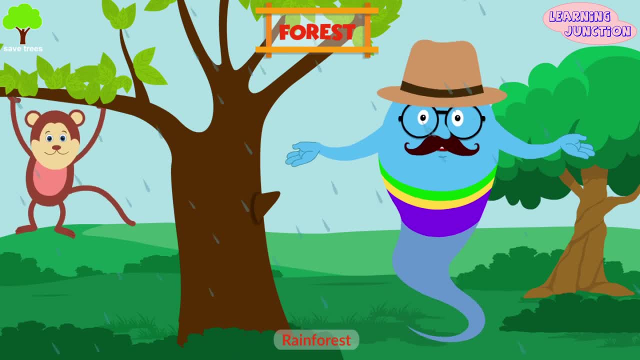 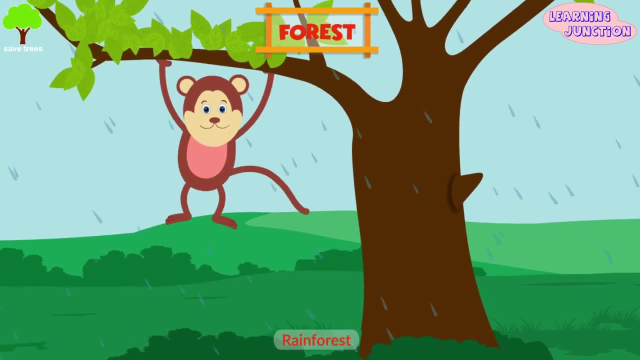 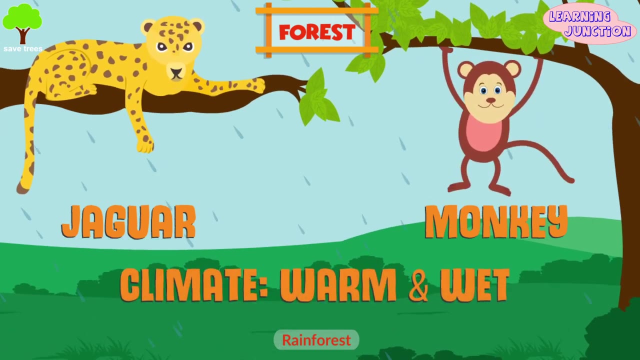 the temperate forest and the taiga. More than half of the world's species of animals and plants are found in the rainforests. Ah, look at that cute monkey. Jaguars and monkeys etc can be seen here. Climate is typically warm and wet. Temperate forests have four distinct 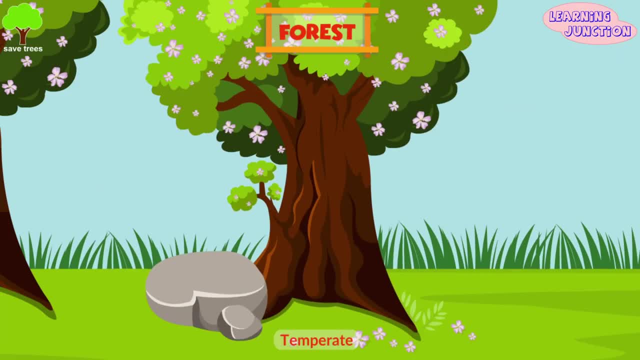 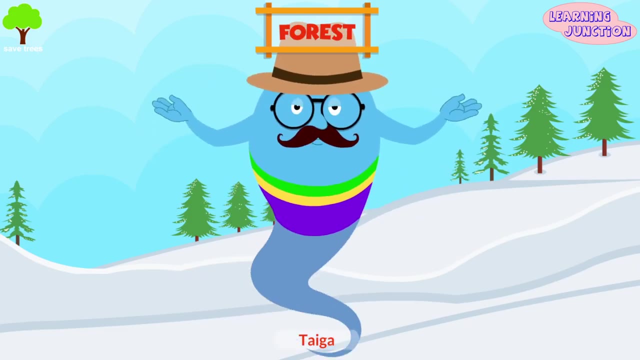 seasons: winter, spring, summer and fall. You'll find various deciduous trees in this biome that lose their leaves in winter and bud new leaves in spring. Raccoons and red foxes are very common in this biome. The taiga is a forest of the cold and sub-Arctic region. Long, severe winters. 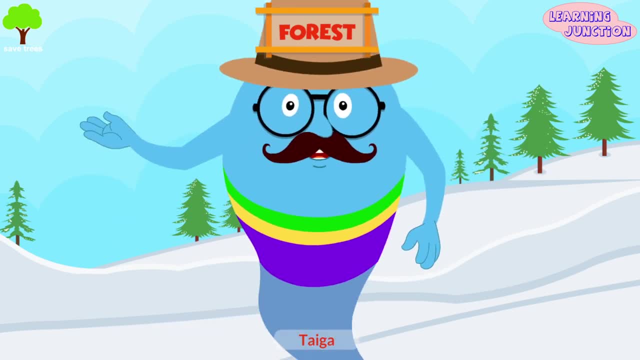 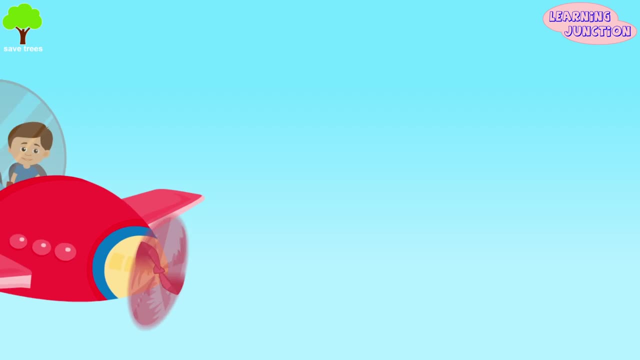 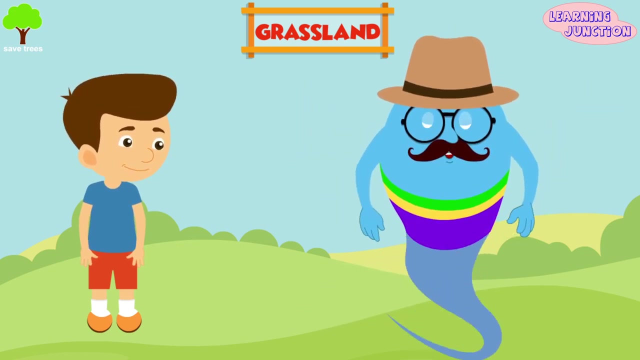 last about six months, with average temperatures below freezing Mammals living in the taiga include bears and squirrels, etc. Let's move towards the grasslands. Grassland biomes are places that receive more rain than deserts, but less precipitation than. 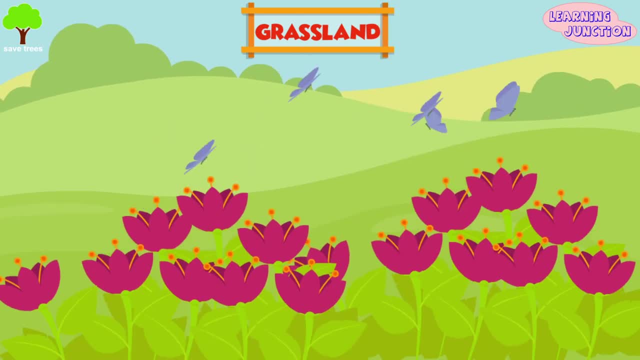 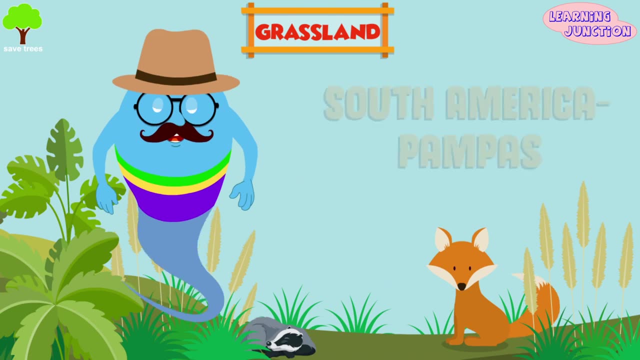 forests. Most of the plants here are grasses and wildflowers which don't need much water. In Africa grasslands are called savannas And in South America they're known as pampas. The largest grasslands are in eastern Africa. In West Africa these are grasslands of the north. the